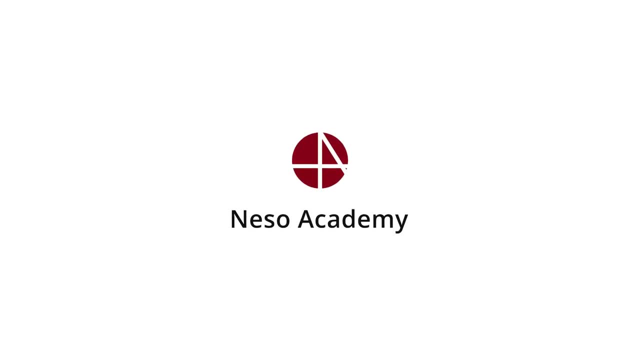 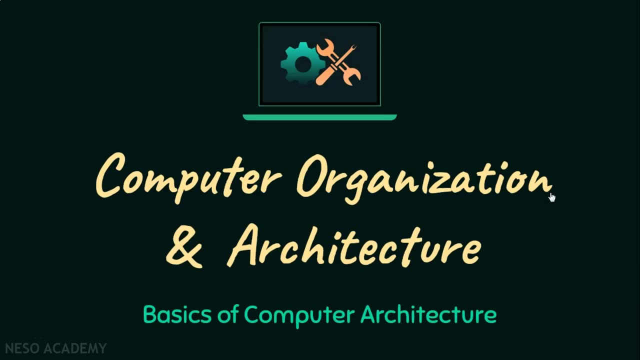 Hello everyone, welcome back to today's lecture of computer organization and architecture. So today we will be learning about computer architecture in a bit details. So let's get to learning. Let's start with the formal definition of computer architecture. So it's. 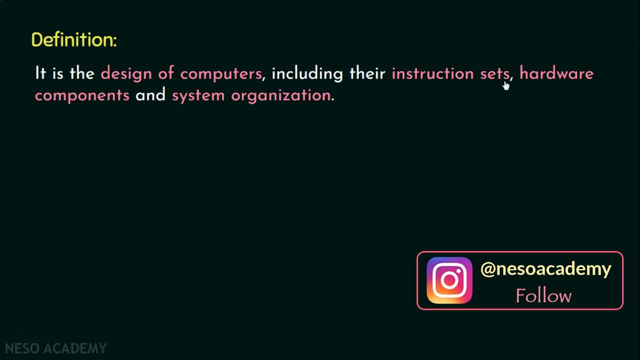 basically the design of computers, including their instructions, its hardware components and system organization. Now it has got two parts. First, the instruction set architecture, which includes the specifications that determine how machine language programs will interact with the computer. Next we have the hardware system architecture, which deals with the 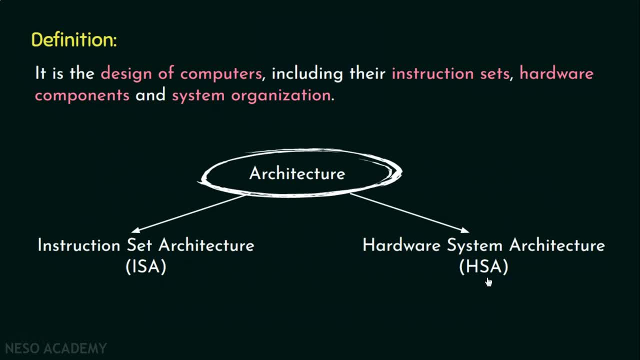 computer's major hardware subsystems like CPU, storage, input-output, etc. It includes both the logical design and the data flow organization of the subsystems and hence determines the efficiency of the system. Let's try and understand this concept with the help of an illustration. Suppose we want 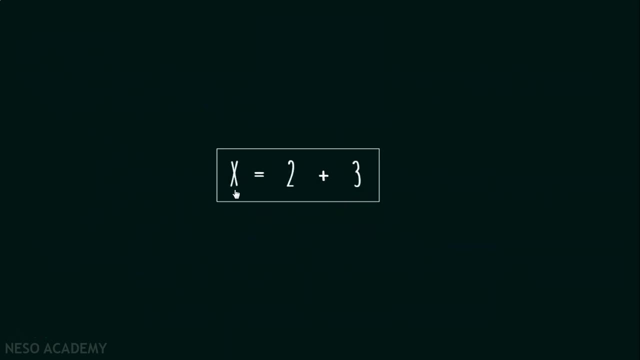 to add two values, 2 and 3, and store the added value in a variable named x. Now this simplification can be performed in various ways, based on the available hardware. These are some examples of the different ways this simplification can be performed. Now, from these one or 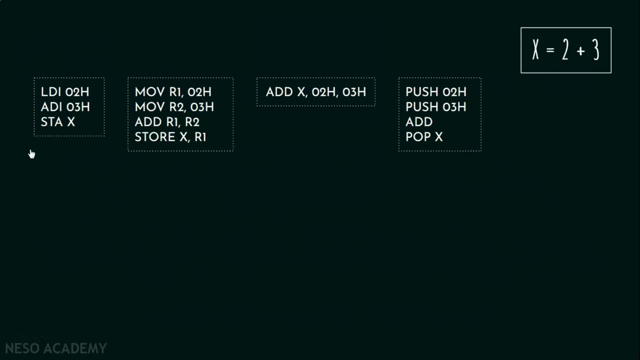 more ways can be selected for a specific type of computer. This is nothing but the ISA. Suppose. this one is selected, So all the other operations will also have similar type of instructions. Now, based on this, the hardware will be chosen, As in this specific case, we will need at least two different. 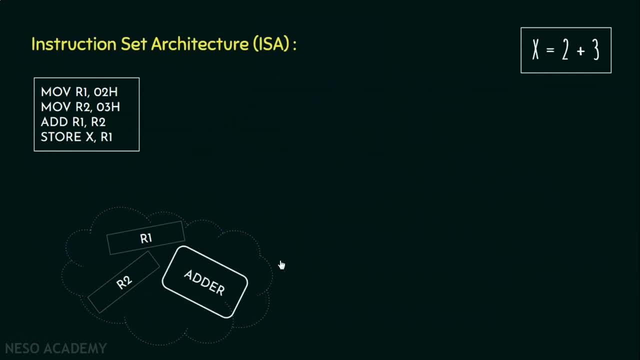 memory locations and an ADAS circuit. It is the rudimentary concept of Hardware System Architecture or the HSA. Now it's really important to distinguish a computer's architecture from its implementation. I hope it was also clear from our previous discussion that the implementation is the 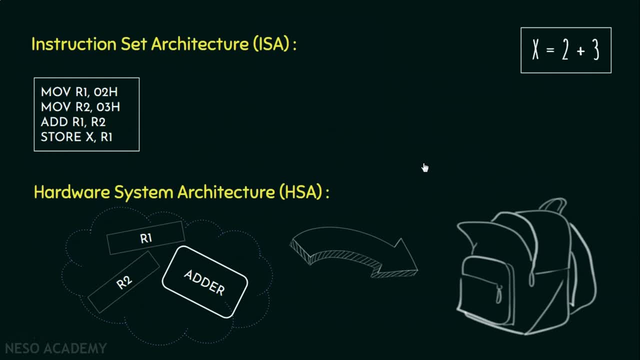 realization of a computer in hardware And includes the choice of technology, speed, cost and so on, Whereas the architecture doesn't really define an implementation. yet they both influence one another. Generally, computers with the same ISA will run the same kind of programs and are also said to belong. 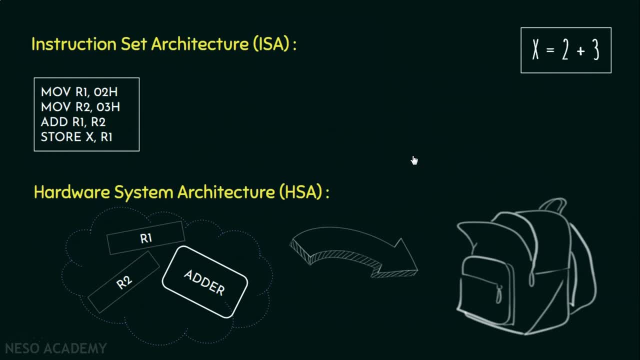 to the same family. This concept will be more clear as we progress. eventually. Now we will move on to the classifications of computer architecture, but before diving straight into it, a bit of a history lesson is required so that we can properly understand various nomenclatures. 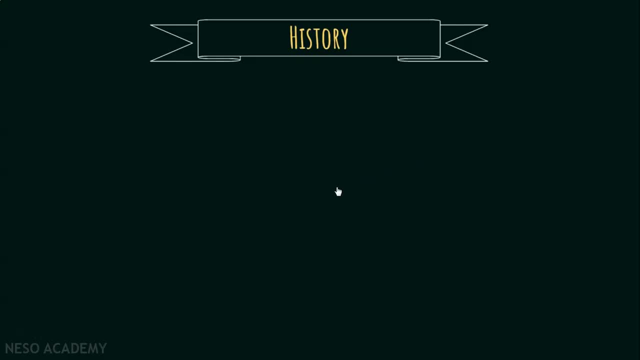 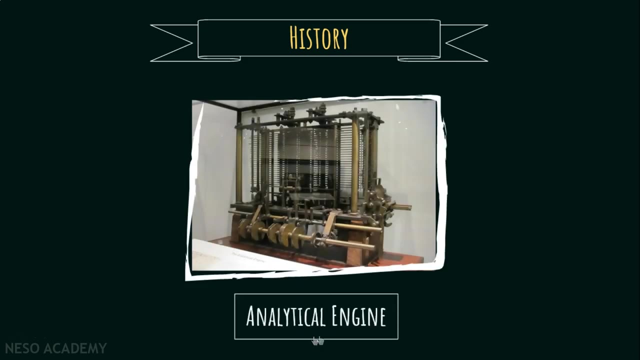 Now we already know that computer architecture is the design of computers, And the great, great, great ancestor of today's ultra-modern computing devices was the analytical engine. It was the first proposed mechanical general purpose computer, designed by the great computer pioneer Charles Babbage. He was assisted by Lady Ada Lovelace, who was the first one. 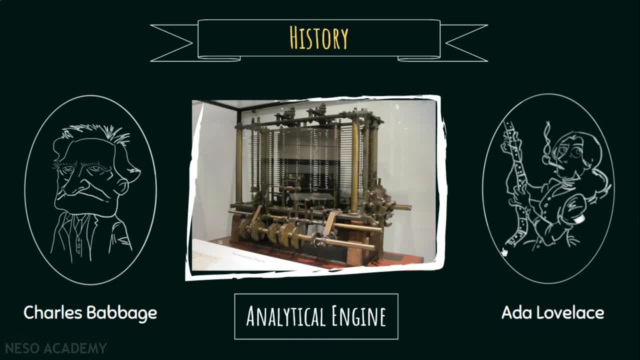 to come up with the basic idea of having a language in order to operate the proposed machine. So, all the ladies out there, more power to you. If it was not for Lady Lovelace, we wouldn't be enjoying the luxury of software today. 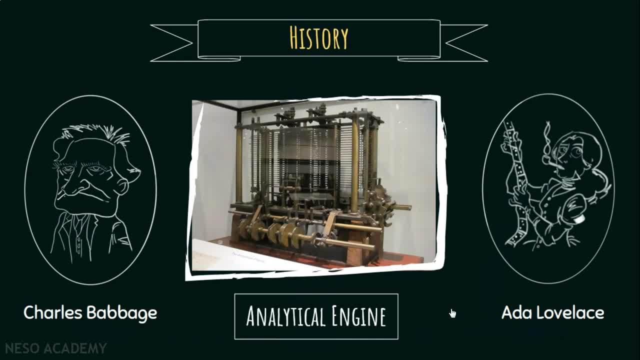 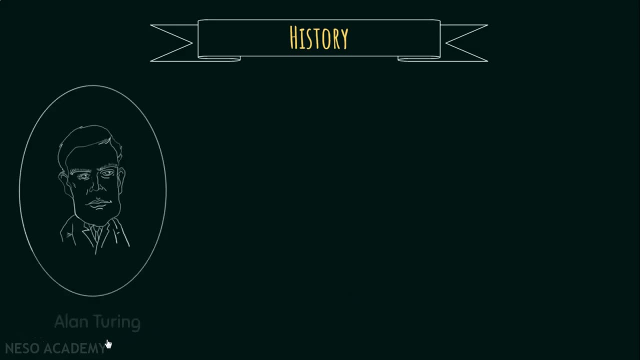 And just an FYI, Lady Lovelace was tutored by the Dee Morgan Augustus. Dee Morgan whose Dee Morgan's law brought revolution to the world of Boolean algebra of George Boole. We all know about that right. Then comes the next big milestone: the advent of computability and non-computability. 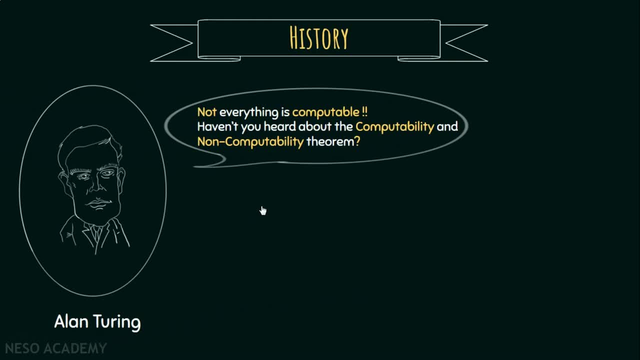 Alan Turing figured it out which problems can be solved using computers. He has widely been considered as the father of computer science and artificial intelligence since then. Now, alongside Turing, another name is very frequently associated with computation, And it is Johann von Neumann, or more popularly known as John von Neumann, This very Hungarian. 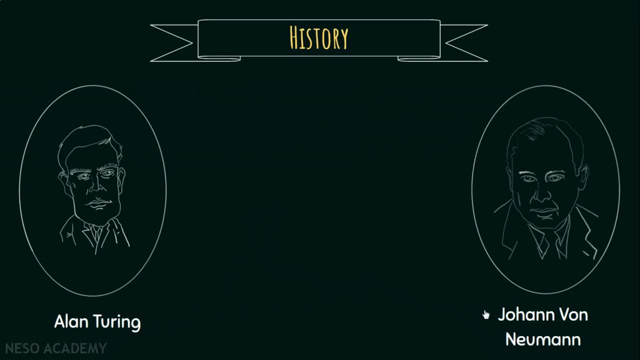 genius was not only a child prodigy who could divide an eight-digit number by another eight-digit number within just a second, But he was also a mathematician who grabbed the full-time professor position at Princeton University by the age of probably 30.. Yes, you heard me right: Not a reader, not a lecturer, but a full-time professor by the 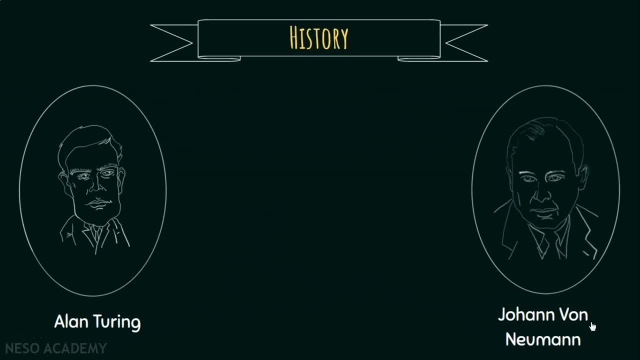 age of 30.. Funny story: Neumann even offered Turing for research assistantship, under his supervision, in quantum mechanics at the Institute of Advanced Studies, where only the greatest of modern minds were invited to work. Also, after the Second World War, Neumann brought together